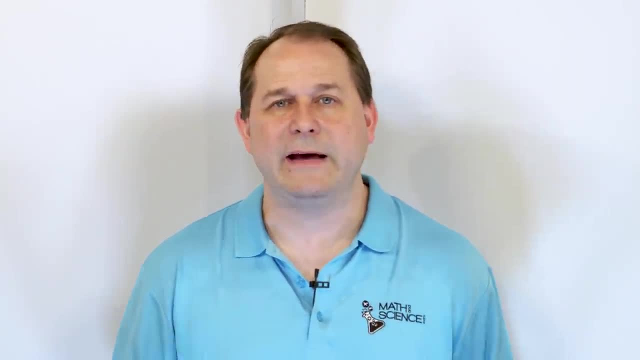 and he says there's a 50% chance of rain. it just means there's about a half half of the chance, half the time it's going to rain and the other half is not going to rain. It's right in the middle. If there's a 0% chance of rain, it will definitely not rain. And 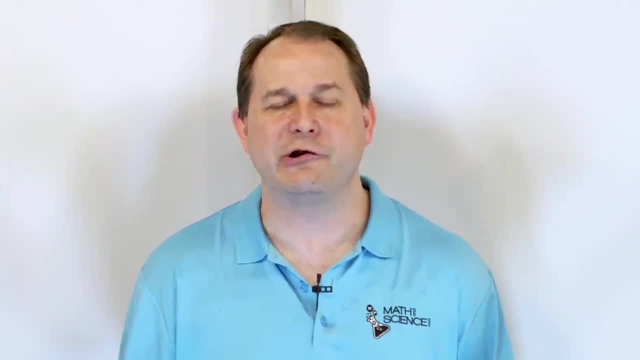 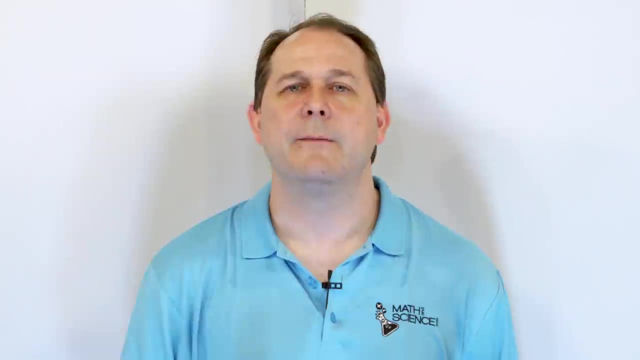 if there's a 100% chance of rain, it's going to rain for sure, But 50% is right in the middle- it won't rain And the other half of the time it will. we're really don't know what's going to happen, but at 50% it's about even as far as like what is actually going. 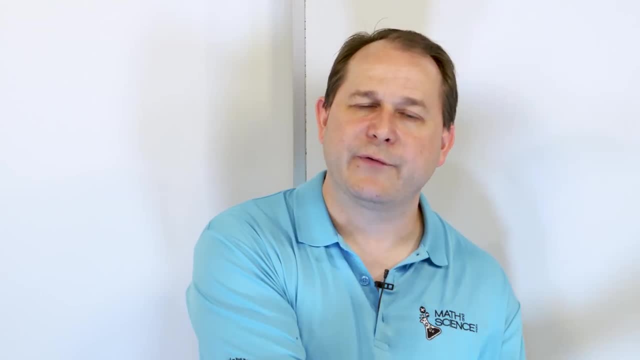 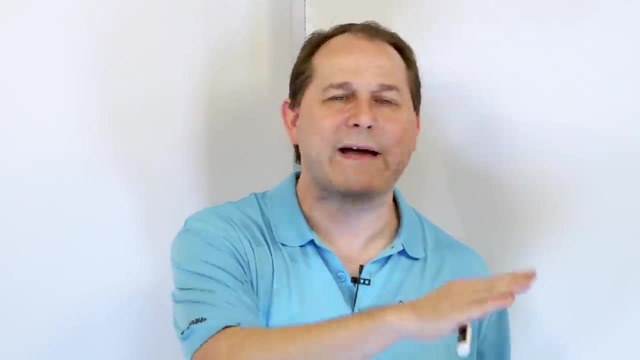 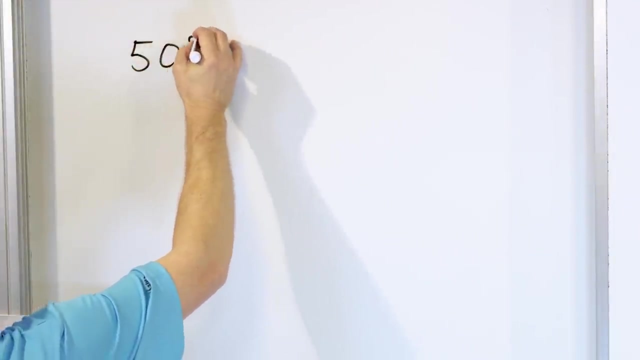 to be the outcome. So we know that percents range from zero on the low end all the way to a hundred on the high end. Let's talk about how to calculate and represent percents when we have any percentage that we're really talking about. So let's talk about this idea of 50%. 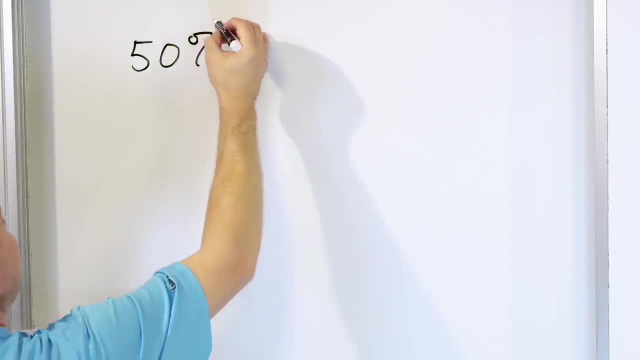 This symbol. you might have to practice writing it a few times. You kind of make a little circle and you come down And you draw another circle. This means 50%. What it literally means is 50 as compared to 100.. Doesn't that sound familiar? We've been talking about ratios, So now we learn. 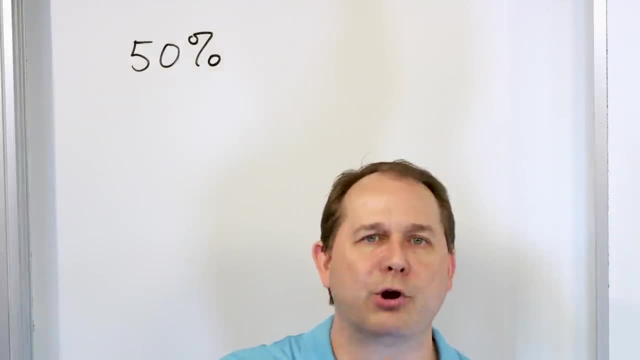 percentages because they're just a type of ratio. Percent means per 100.. All right, So we write percent like this. If I say give me 50% of your money, I tell you this. If I say the price of the uh of the watermelon is 50% off, I write it like this. That means: 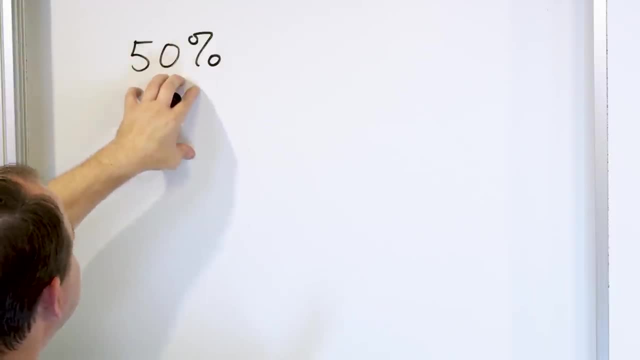 half off. If I say it's going to rain with a 50% chance, this is how I write it. If I say it's going to rain with a 50% chance, this is how I write it, But there are other. 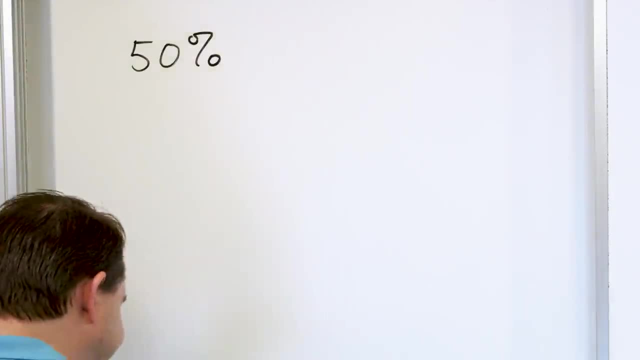 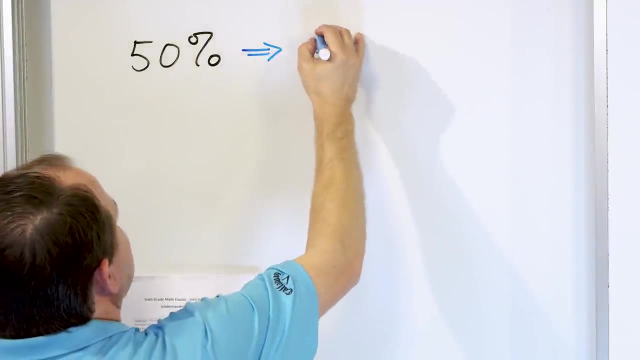 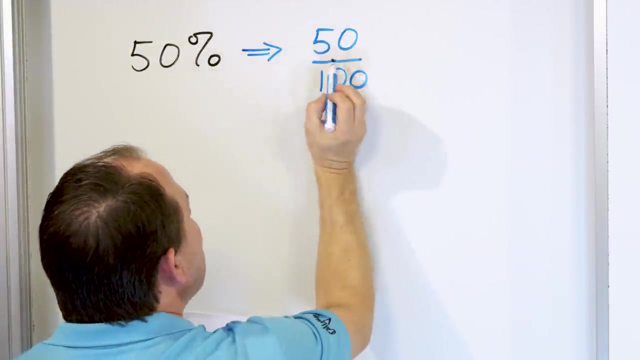 ways to write percentages right. What does a percent actually mean? 50% actually means that it's 50 as it compares to 100 because, remember, percent, this symbol means per 100. So 50 per is the line and 100 is down here, So this symbol means per 100.. So this thing. 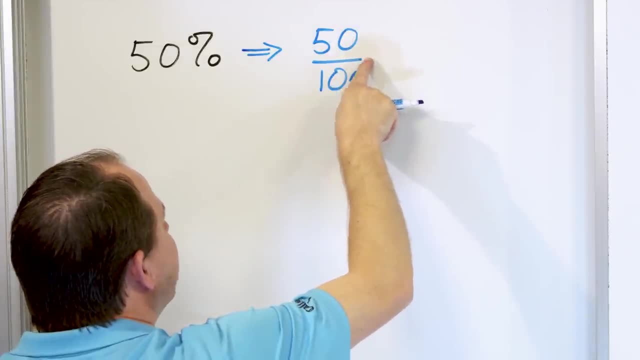 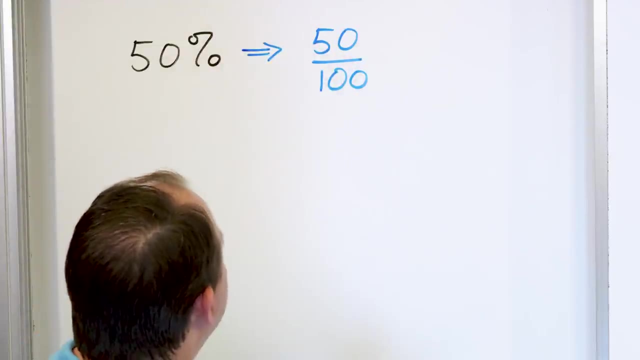 means exactly the same thing is 50 divided by, or fraction bar 100. So let's talk about what would happen if we actually did this division: 50 divided by 100.. So what we're going to do is I'm going to divide it for you the first time and then 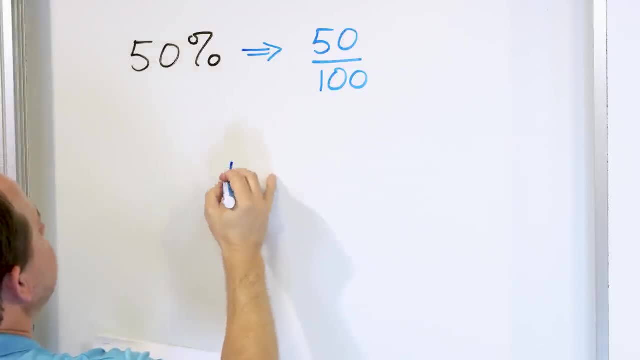 I'm going to show you the simpler way to do it. Let's take 50 and let's actually divide it by 100, because this is what it is: It's a division, or fractions are all division, right? So notice, you have a 50, you have an invisible decimal point here at the end. Um, 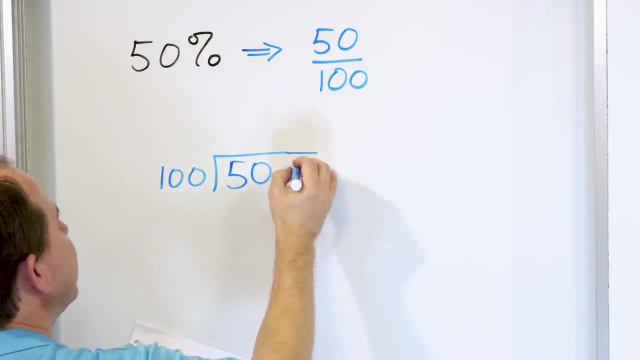 and so we're going to say: how many times can a hundred go into 50?? It can't, So we're going to drop a zero at the end. How many times can? and don't forget, your decimal is going to float right above there. 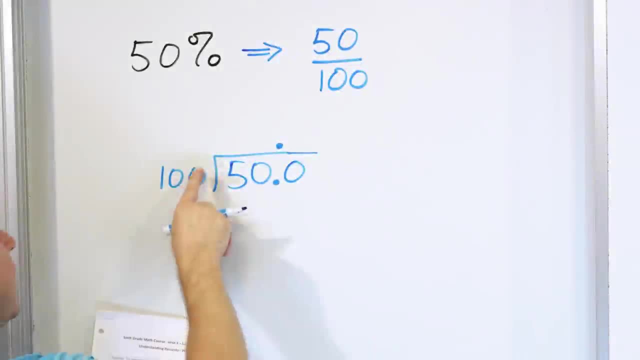 How many times can 100 go into 500?? So 100 times something is 500. There has to be a five here, And when you multiply you'll get 500 and you'll subtract, you get a zero. So we can basically stop because, uh, we've got a remainder of zero. What we figured out is: 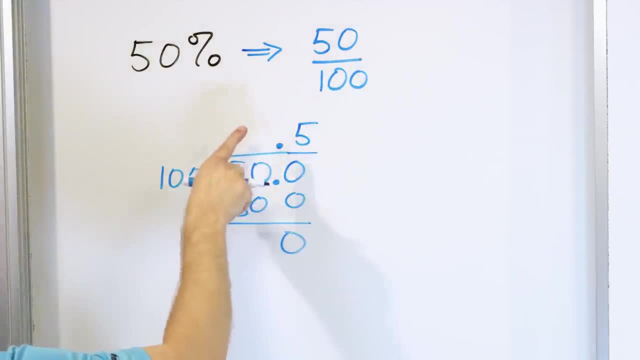 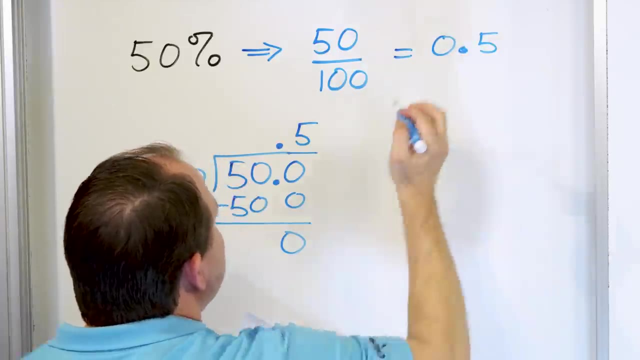 if we take 50 and we divide it by a hundred, the answer is 0.5, which is another way of writing 0.5.. So what we're trying to show you is that there's different ways to represent percentages. Every. 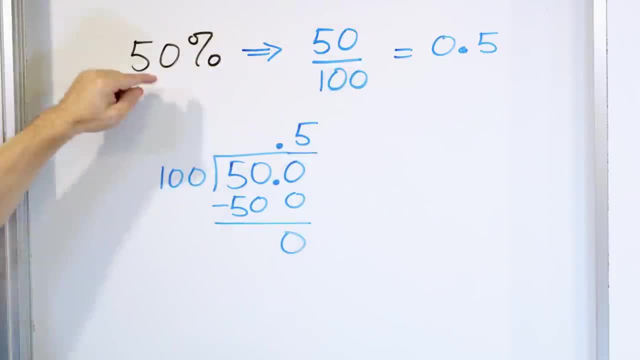 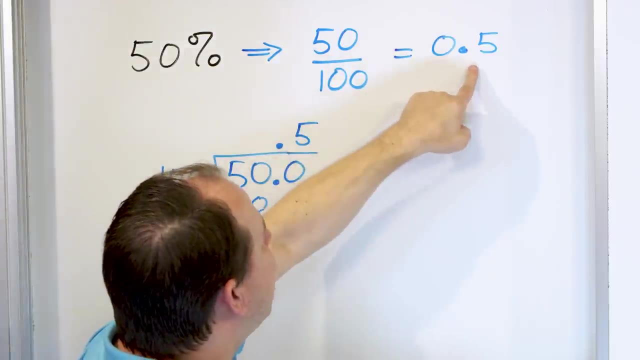 percent can be converted to a decimal, And the way you convert it is: you take the 50 and you just divide it by 100, because that's what percent means. And when we do this division we figure out that the decimal equivalent of this thing is 0.5.. So this is another way. 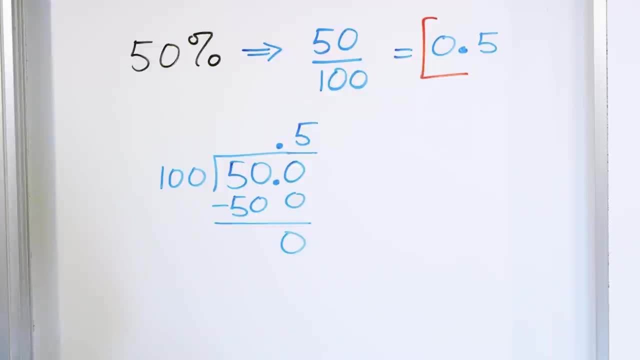 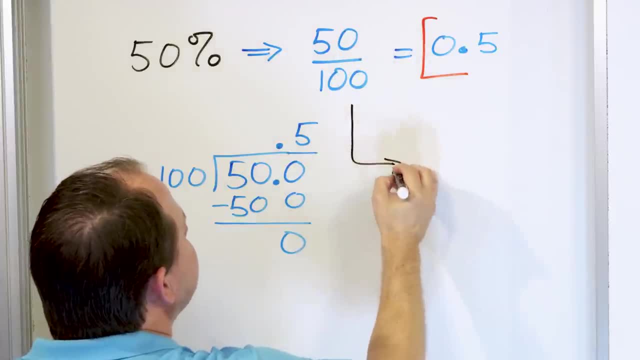 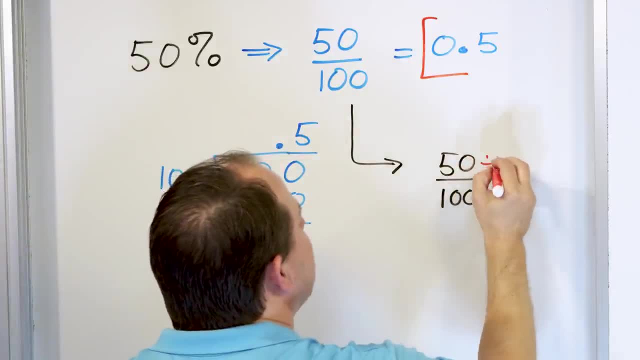 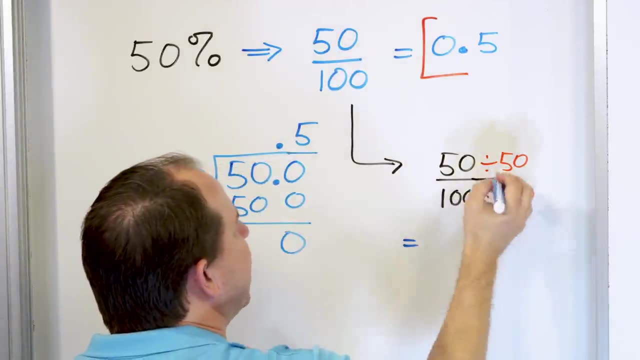 50 on the top and 50 on the bottom. I can simplify it: I can divide the top by 50, and the bottom also by 50. And what will I actually get? 50 divided by 50 is 1, and 100 divided. 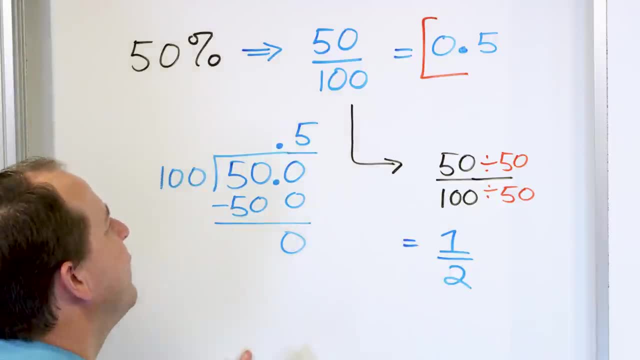 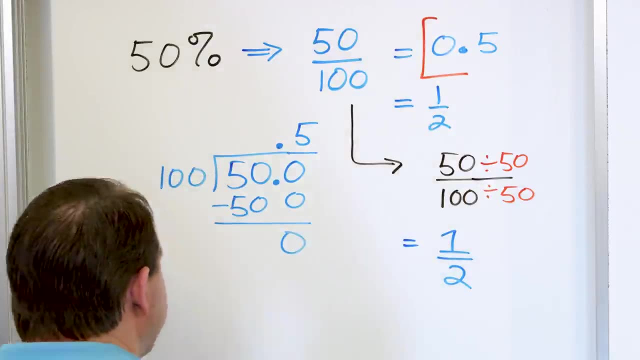 by 50 is what 2.. So I get an answer of 1 half. So up here I will also say that this is also equal to 0.5.. to 1 half. So, putting it all together, what we have figured out is that this: 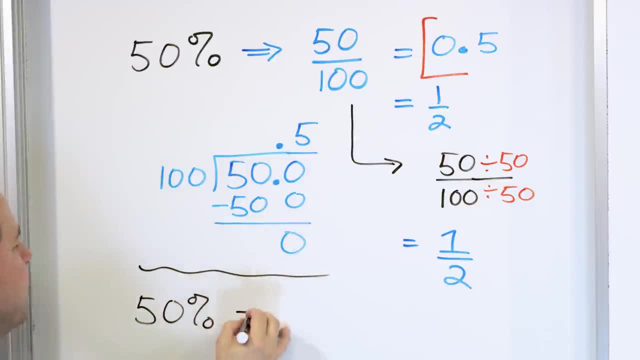 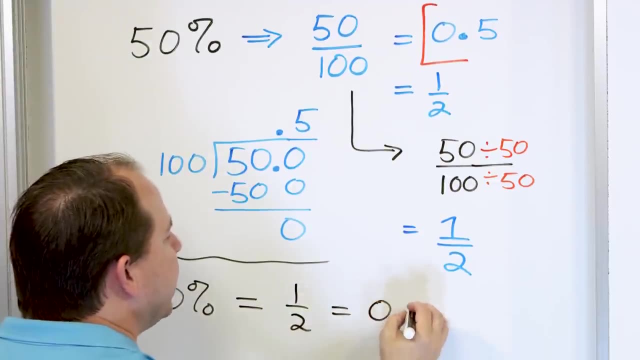 percentage, which is 50%, can be also written as the fraction 1, half right, And then you can also write it as a decimal, 0.5, and all three of these are the same way of saying the same thing. It's important for you to know that every 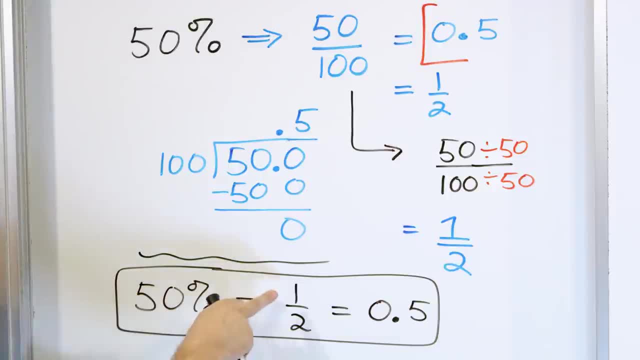 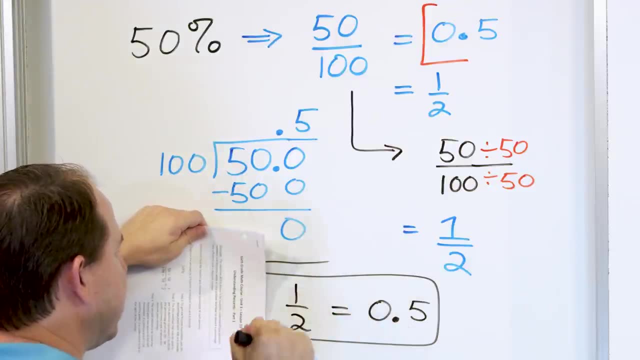 single percentage can be converted to a fraction, which can also be converted to a decimal, and these all mean the same thing. In the past, we have learned about fractions and you can convert them to decimals. We learned that. Now you're learning that you can also represent all of these as a fraction. So if I tell you, 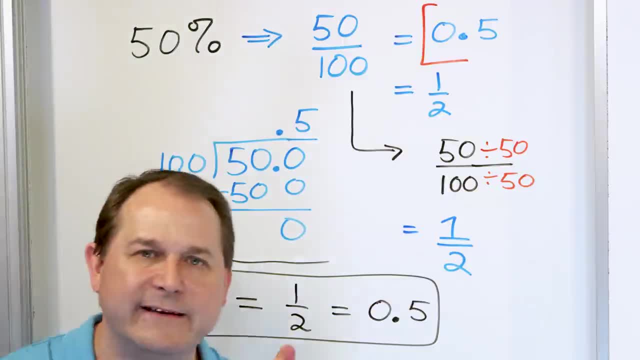 it's gonna rain tomorrow with a 50% chance. that's the same thing as telling you that half the time it's gonna rain and half the time it's not, which is another way of saying 0.5.. If you think of a scale of 0 to 1, then 0.5 is. 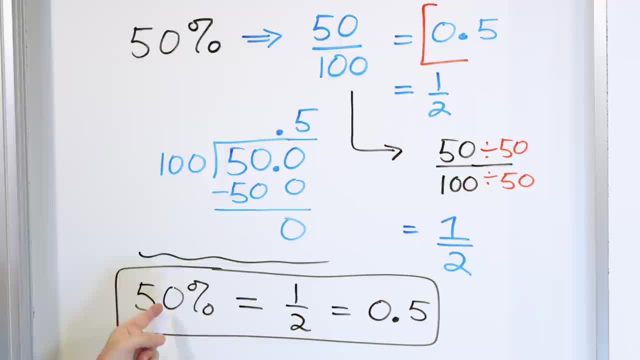 right in the middle. So, whereas this is on a scale of 0 to 100, 0.5 is right in the middle. So, whereas this is on a scale of 0 to 100, 50% is right in the middle. This is a scale of 0 to 1, 0.5.. So the 0.5. 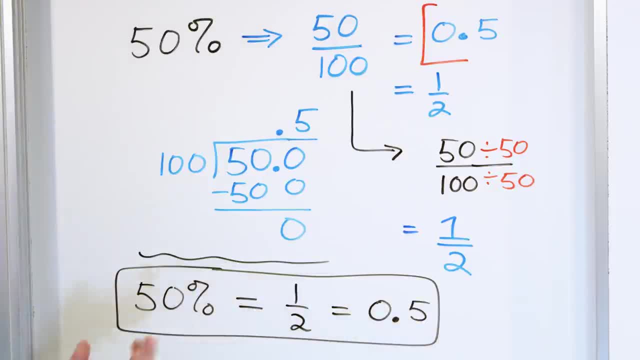 means the same thing as 50%, and the one-half means the same thing as well. Now, the last thing I'm going to tell you before we move on to the other problem is we took 50 and we actually divided it by 100. And I did the long division to. 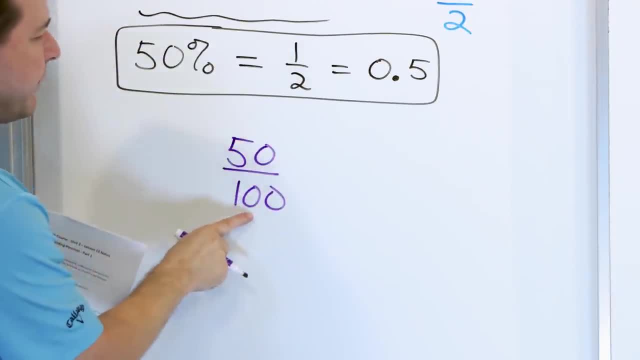 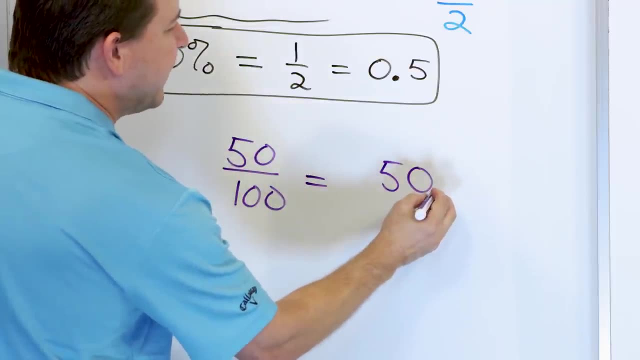 show you, but I want to remind you that when you divide any number by 10 or 100, there's a much simpler way to do it. All you do is you remember that this 50 always has an invisible decimal point at the end. All numbers do, And when I 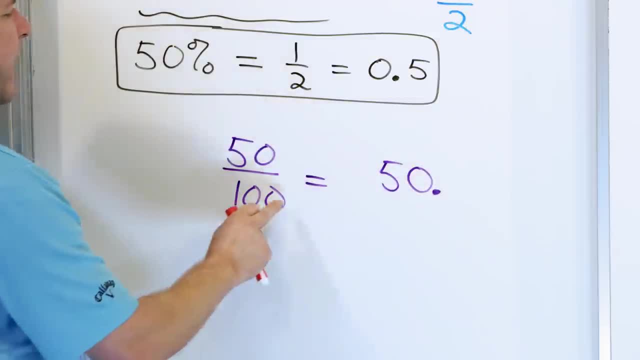 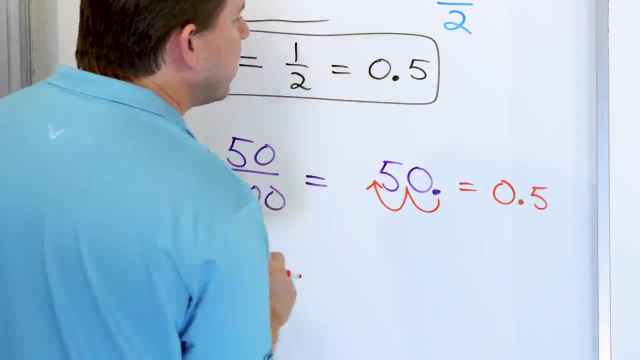 divide just by 10, I move the decimal one spot to the left, And when I divide by 100, I move the decimal two spots to the left. So 0.5, right Or 0.50.. It's the same. 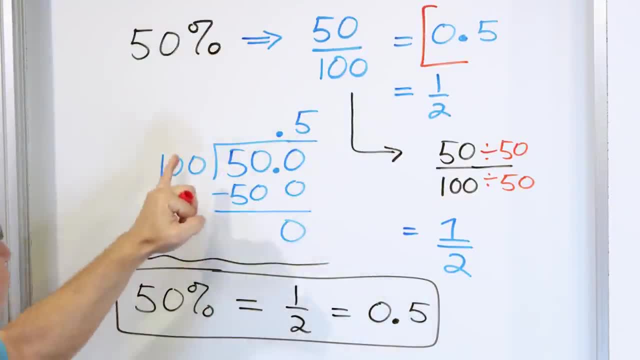 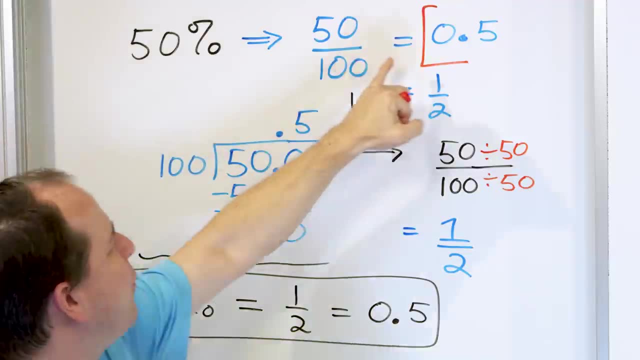 thing. You put a zero at the end. So instead of doing the long division when I convert to a decimal, all I'm gonna do is move the. since I'm dividing by 100 every time, I'm gonna move the decimal two spots to the left. That will always. 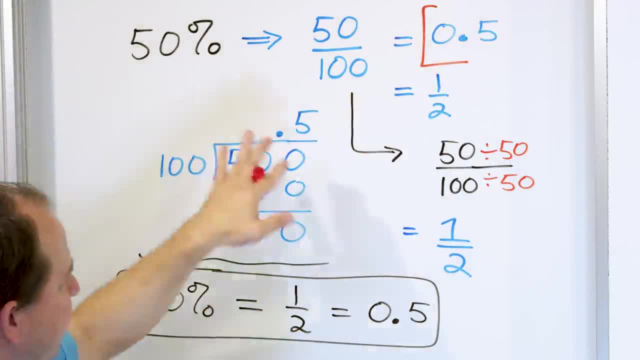 be the decimal equivalent of 100.. So I'm gonna move the decimal two spots to the left. That will always be the decimal equivalent of 100.. of that, And then to convert to a fraction, I'm gonna do the same thing I've done here. So I just wanted to point that out to you because it's gonna be. 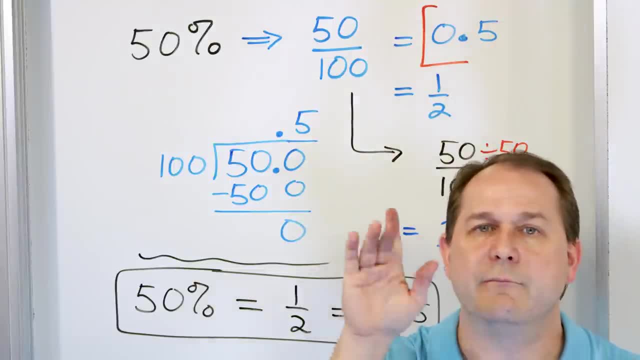 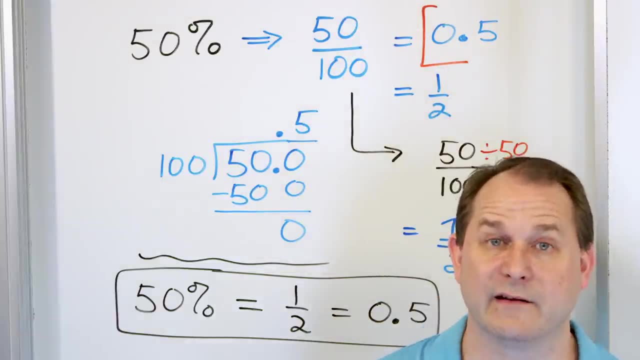 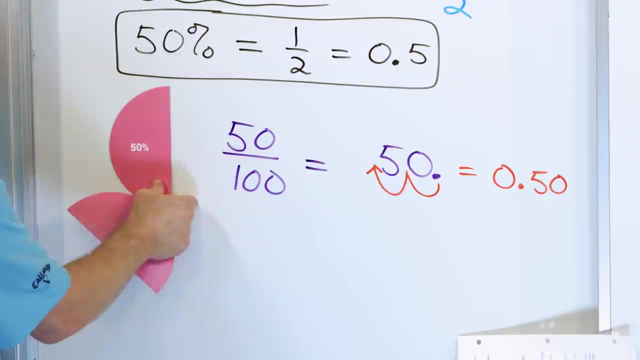 much, much easier for you to just move the decimal instead of actually doing the long division, because we're always dividing by 100. So we're always gonna move the decimal two spots to the left. So let's see what this actually means. What we're saying is that we were talking about a 50% right. Notice that we. 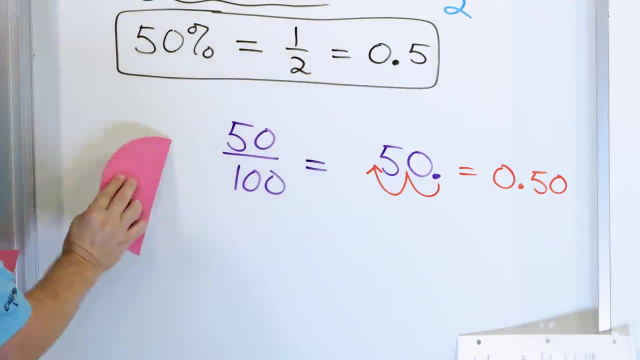 said it was equivalent to one half. We said one half, So this is half of a pizza and this is another half of a pizza. Together they make a whole pizza. right? We're saying that one half is exactly the same as 50% And lo and behold, if you flip these guys over half of this. 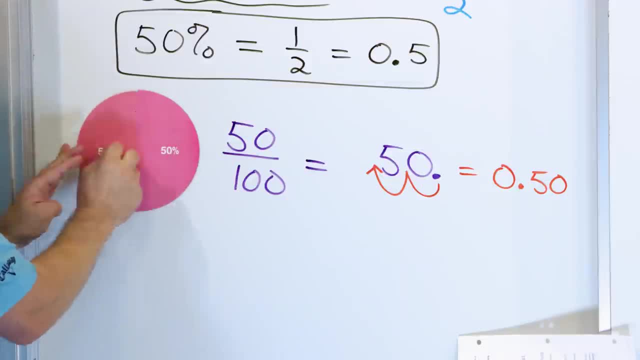 pizza is exactly equal to 50%. The other 50% would make the other half of the pizza. So, as before, in fractions you think of part over whole. in percentages you're thinking of part over 100, kind of. So we know that if you take 100, 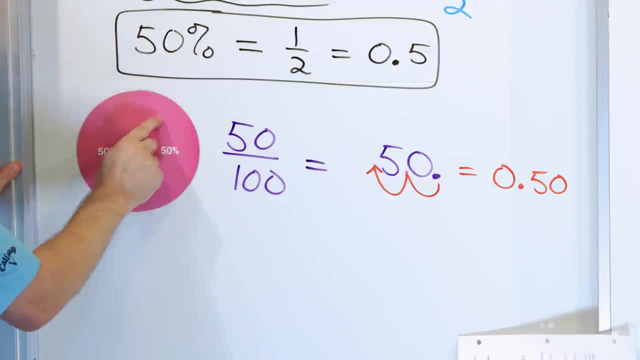 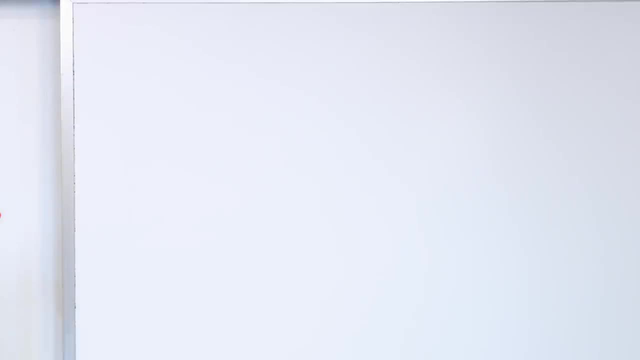 divided by two, you get 50. So this half has to be 50%, and this half has to be 50%, just as we've been talking about, a minute ago, Different ways to think about it. Now, the first problem always takes the longest. The remaining problems: 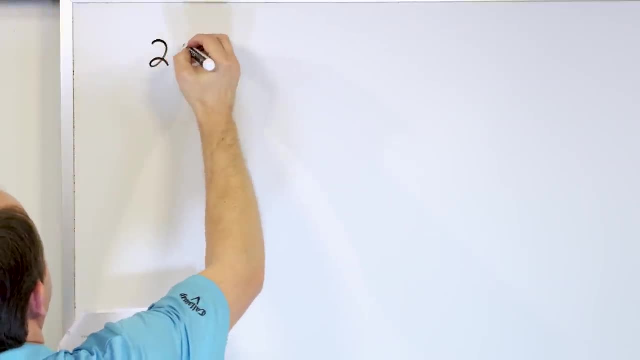 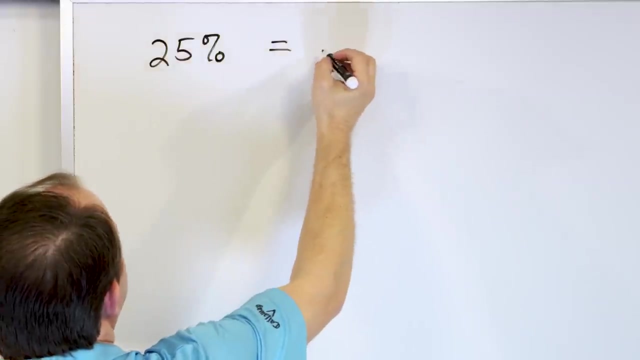 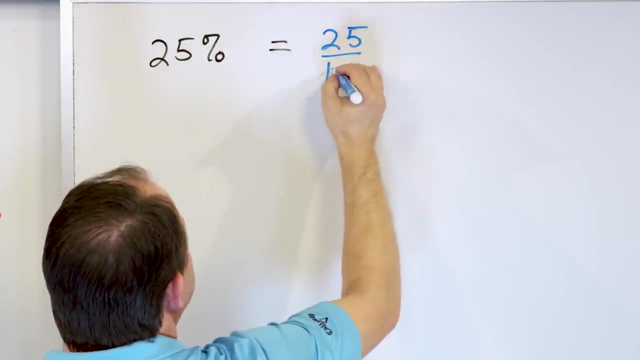 are going to be much, much faster. Let's represent the percentage: 25%. We want to express it as a fraction, and we also want to express it as a decimal. How do we express it as a fraction? Well, the percentage means 25.. That's what it is, And this means per 100.. So we're 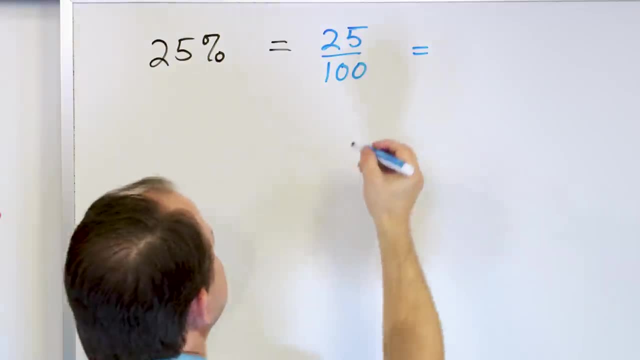 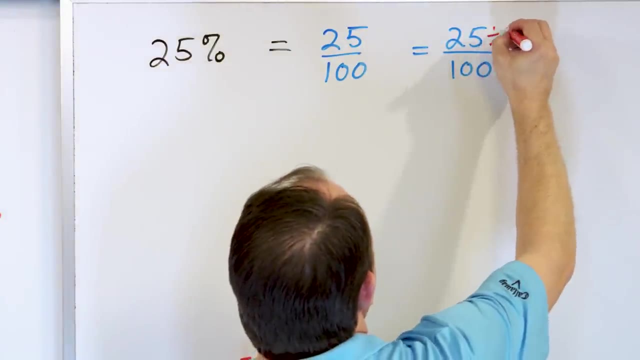 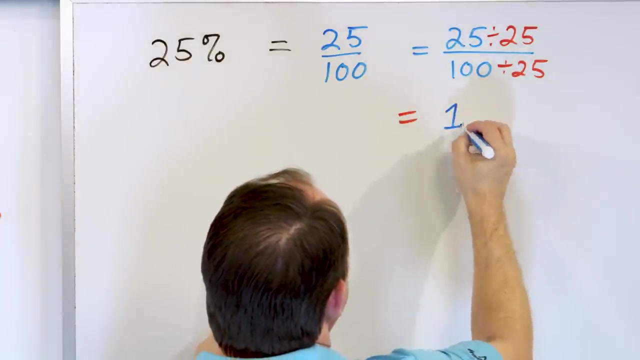 just going to divide by 100. But what we're going to do is we're going to simplify this fraction: 25 over 100. We can divide top and bottom by what. We can divide top and bottom by 25.. Right, So what do we get? 25 divided by 25 is 1, and 100 divided by 25 is 4.. So 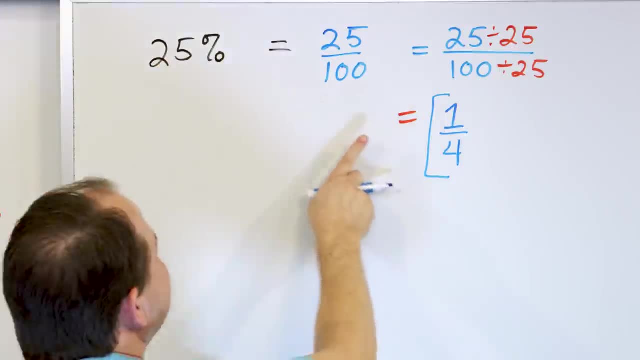 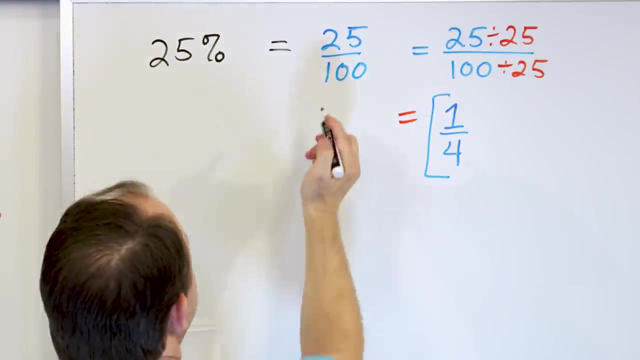 we're saying that the percentage 25% is the same thing as 1 fourth. That's what we're saying Right Now. let's also convert it to a decimal. When we're doing 25 divided by 100, it's going to be faster for us to write the 25 down. 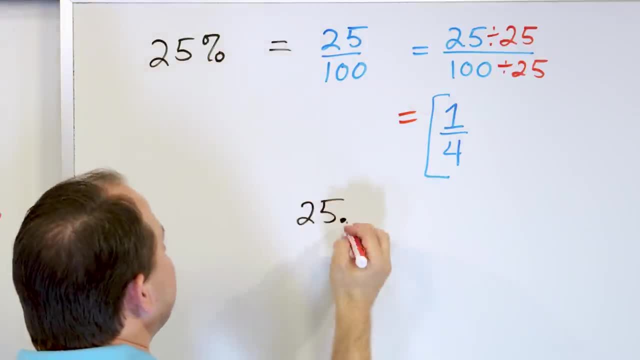 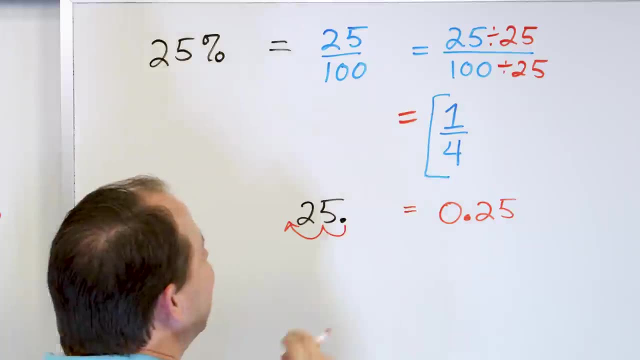 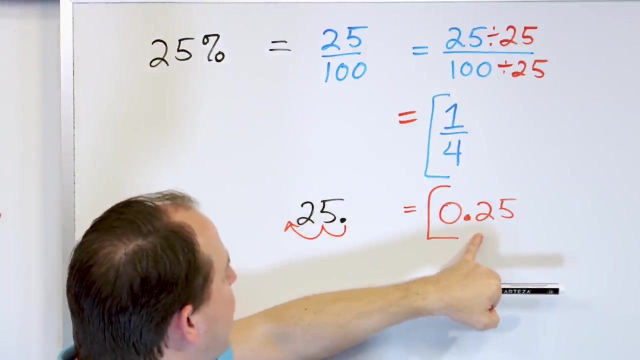 The decimal point is always at the end, And since we're dividing by 100, we move it two spots to the left, And so the answer here is going to be 0.25 as a decimal. So what we're saying is that the fraction 25% can also be written as a decimal- 0.25, and it can. 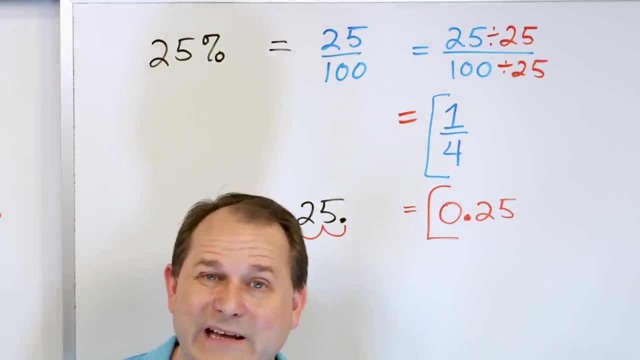 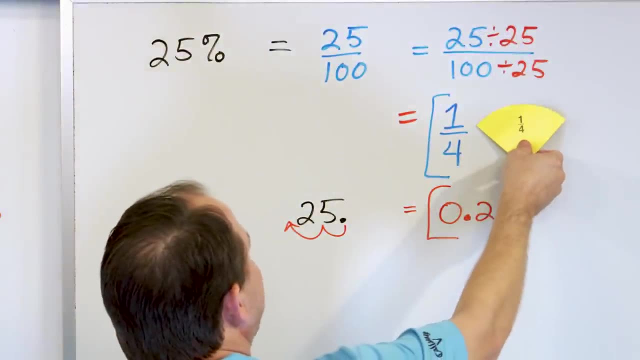 also be written as a fraction: 1 fourth. So we're going to do the same thing. So let's go and take a look and see if we can understand that. So we basically said: 1 fourth is the answer to this. So if we build a pizza out, 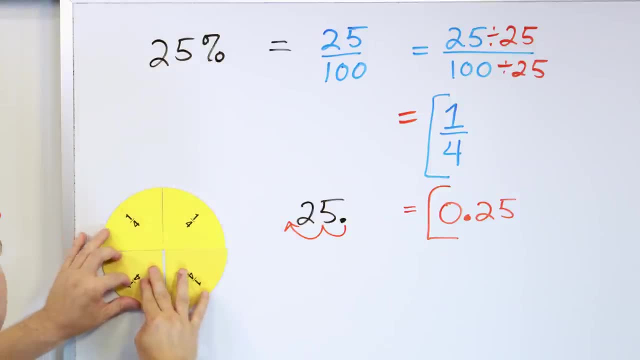 of fourths. here we have 1 fourth, 2 fourth, 3 fourths, 4 fourths. Right, What we're saying is that this 1 fourth is really equivalent to 25%. This other 1 fourth is equivalent. 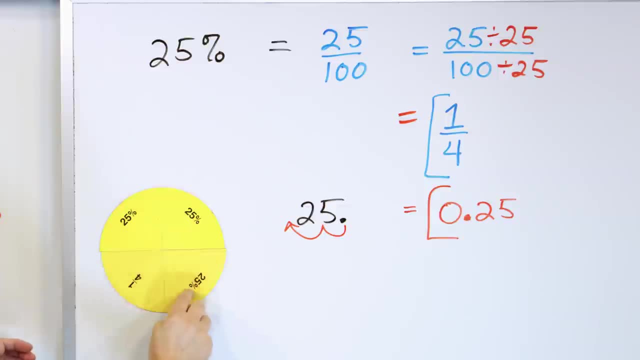 to another 25%. This other 1 fourth is equivalent to another 25%, And then this final 1 fourth is also equivalent to another 25%. Of course, if you add all the percentages up and you get a whole, you should end up. 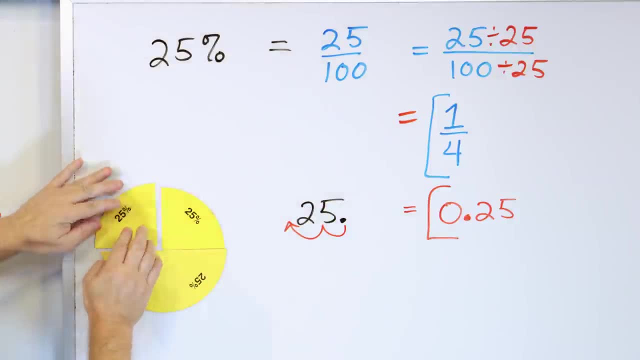 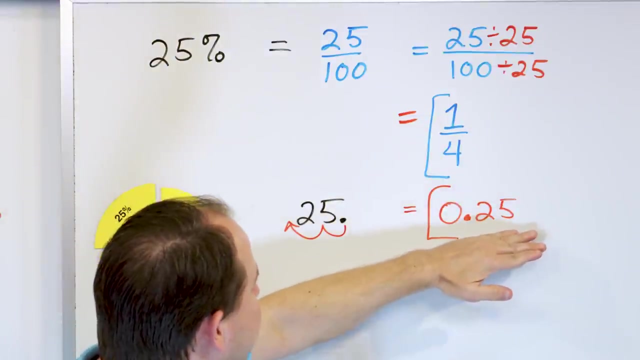 at 100%, And that's what we get. So this fourth over here is worth 25%. here, which is what we basically are: showing you that 1 fourth of a pizza is the same as 25%, And then as a decimal it's just 0.25.. And the reason why we have a decimal equivalent here is because 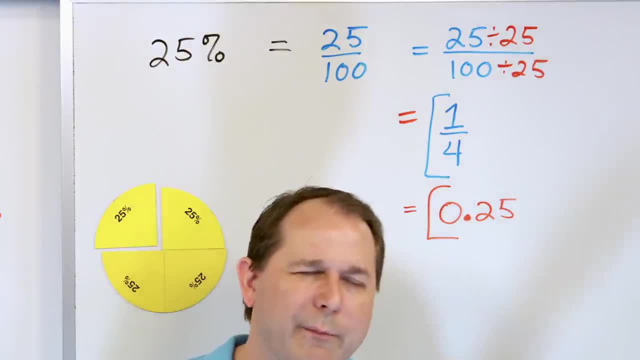 when we're going to multiply by a percentage, we always- almost always- convert to a decimal when we're doing the multiplication. We'll do problems like that a little bit later, But for now, just to know that 25% is the same as 0.25.. Notice, the numbers are the same. 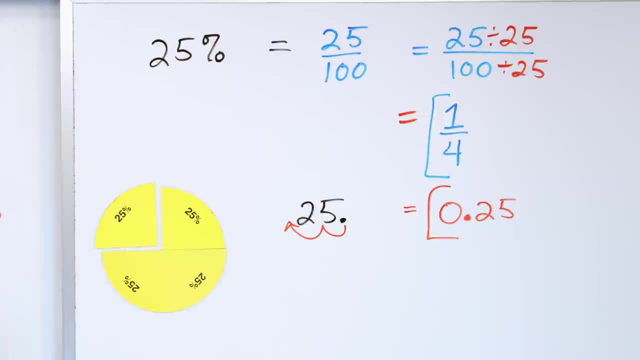 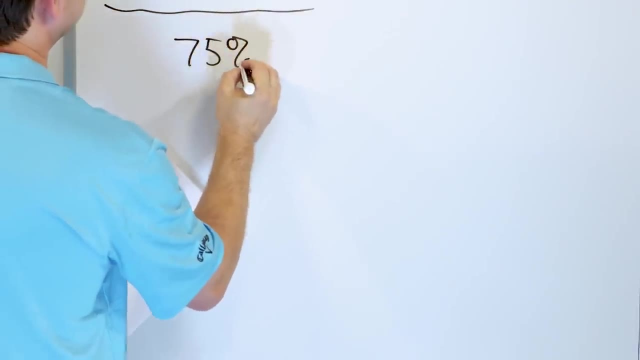 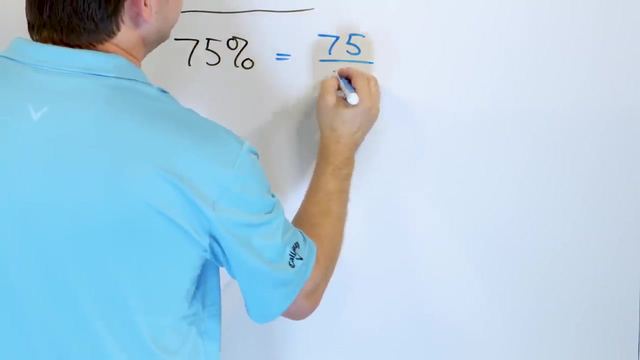 The decimal just moves, which is the same as 1. fourth. All right, Now let's move along to problem 3.. Let's say that we have the percentage 75%. All right, How do we convert it to a fraction, into a decimal? Well, 75% means 75 out of 100.. That's what it means, And I can. 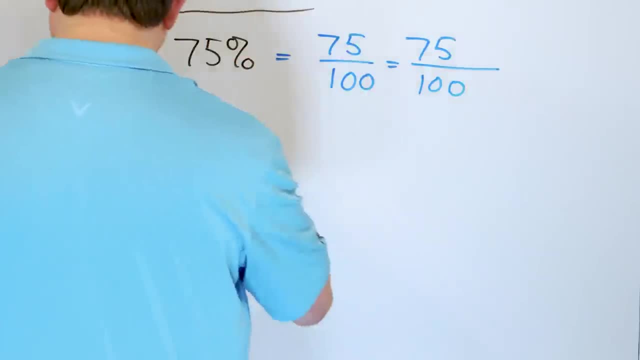 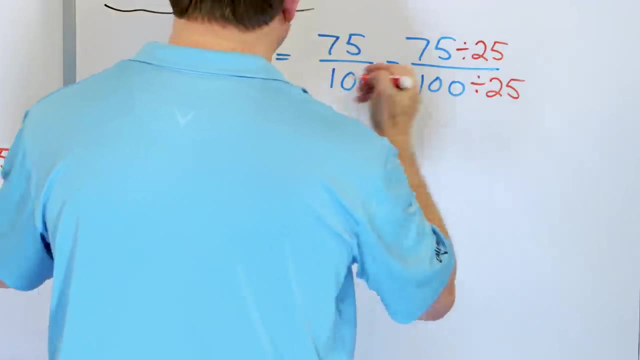 simplify this. So if I get 75 out of 100, I can simplify it by dividing the top by 25 and divide the bottom by 25.. What do I actually get? 75 divided by 25.. If you think 25, and then plus another. 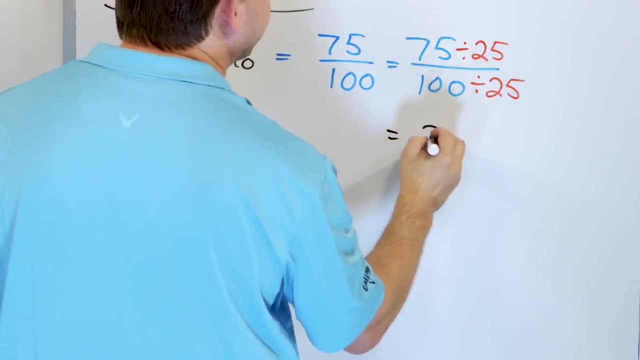 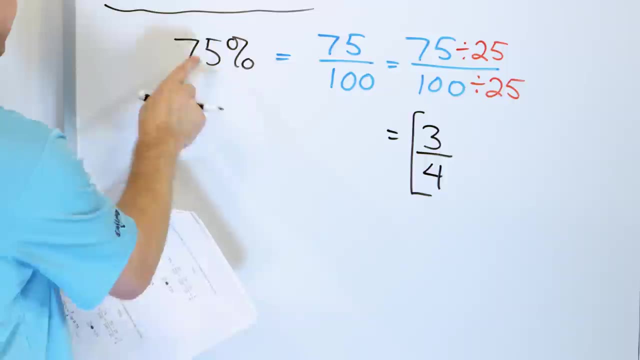 25 is 50 and another 25 is 75, the answer here is 3.. And then 100 divided by 25 is 4.. So the fraction equivalent is 3 fourths for 75%. So we're saying that 75% is the same. 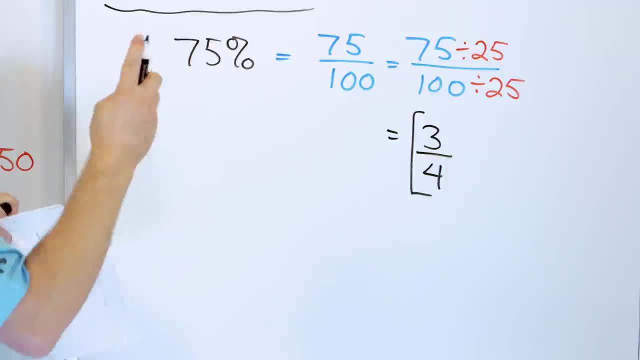 as 0.25. And then what would be the decimal equivalent? Well, if there's an invisible decimal point at the end, then to find the percentage, we just move it two spots to the left, which is 0.75.. You can think of it with the 75, and you have a spot right there and you move it. 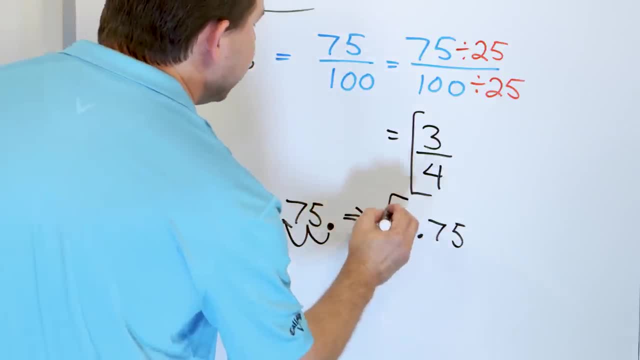 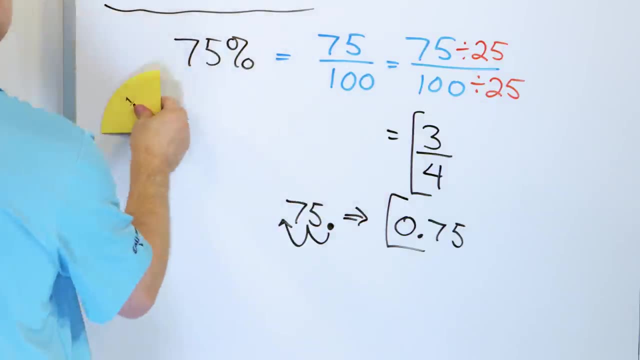 two spots to the left, because we're dividing by 100. And so you get 0.75.. So these are all three the same. Let's see if it makes sense. We're saying that it's equal to 3 fourths. 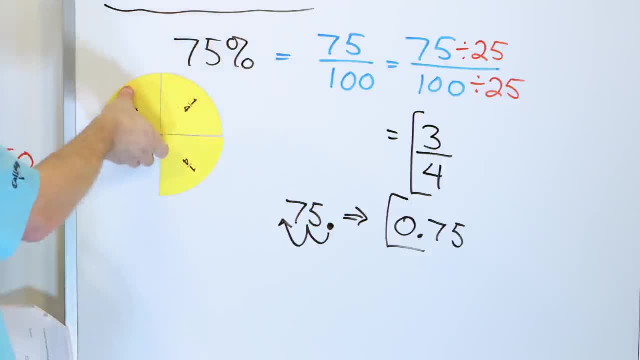 Here's 1 fourth, Here's 2 fourths, Here's 3 fourths, And 1 fourth, we already know from above, is equal to 25%. So there's 25%, And then this next fourth is another 25%, And this final fourth is another 25%. 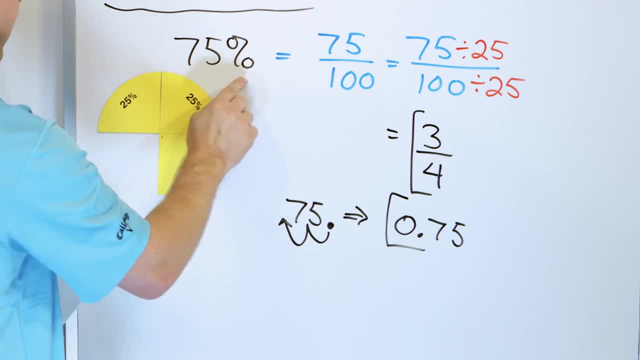 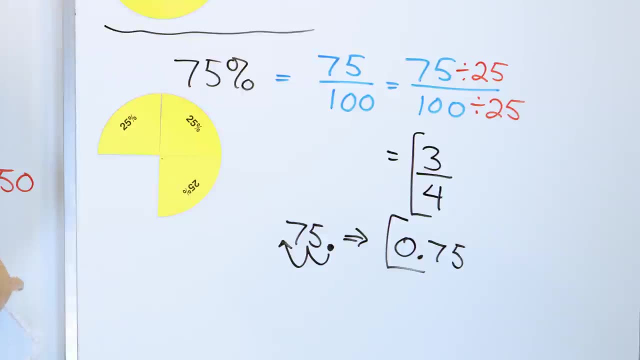 And all together they make 75%. So 75% is 3 fourths, because 25% is 1 fourth. And so if you have 3 fourths, then 25 times 3 is 75. And then the decimal equivalent of this. 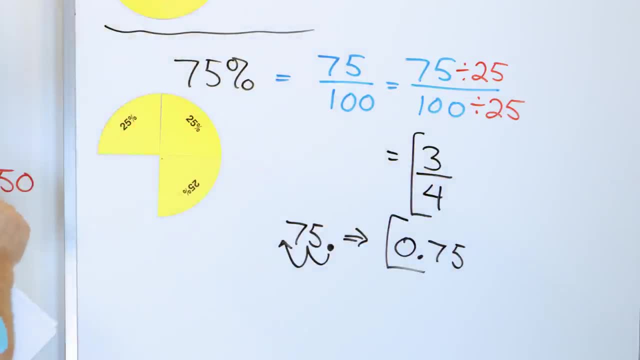 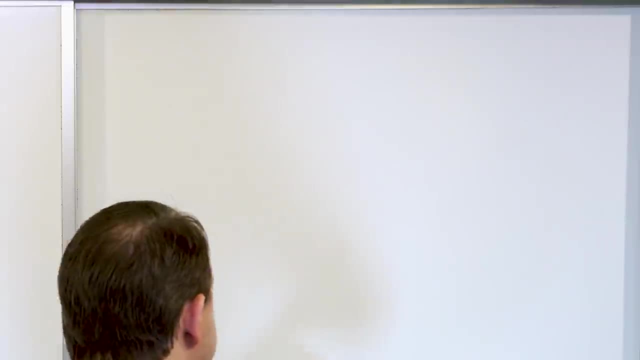 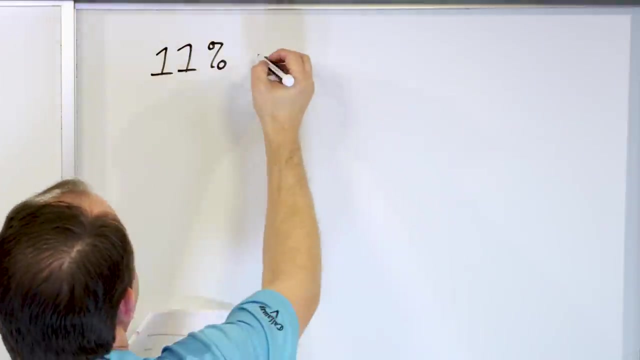 percentage is 0.75.. These are all three the same exact thing. All right, Now we're not going to use any more magnets, We're just going to crank through the remaining problems. Let's convert 11%. Let's convert it to a decimal right: 11.. 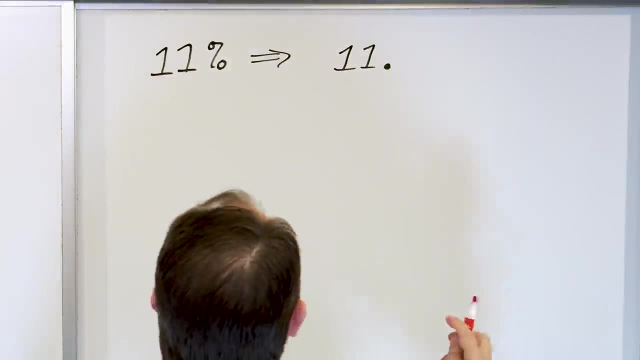 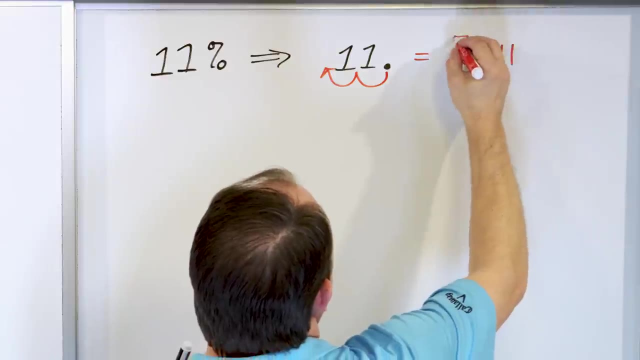 There's an invisible decimal at the end. We're going to be dividing by 100, right, So we move the decimal two spots to the left, which means 0.11.. This is the decimal equivalent of 11%. All right. 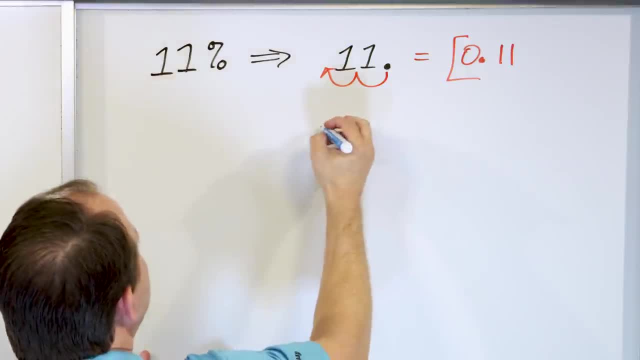 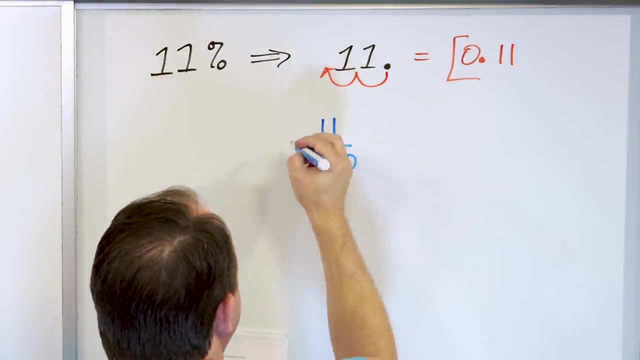 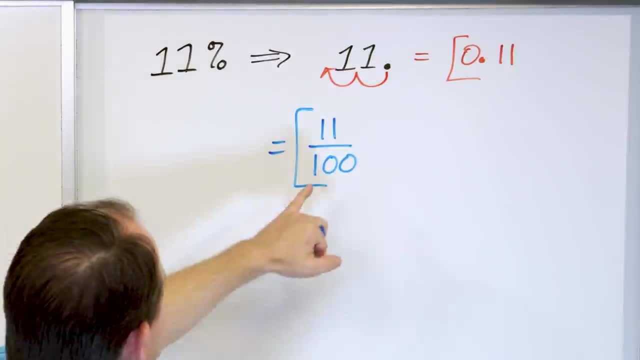 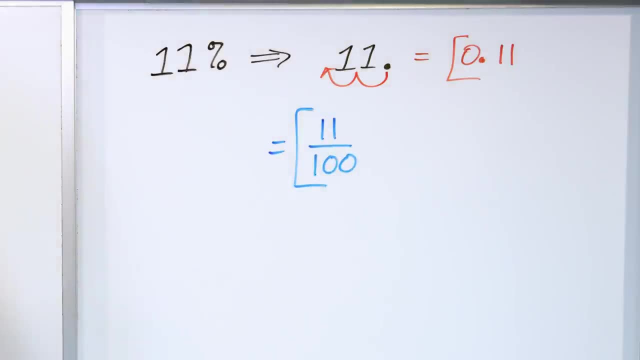 I really am just done. It's just equal to 11 over 100.. And you can see why the decimal is moving two spots to the left, because when I divide by 100, I'm going to move that decimal two times. All right, Next problem: what about 14%? What about 14%? How do I convert that? 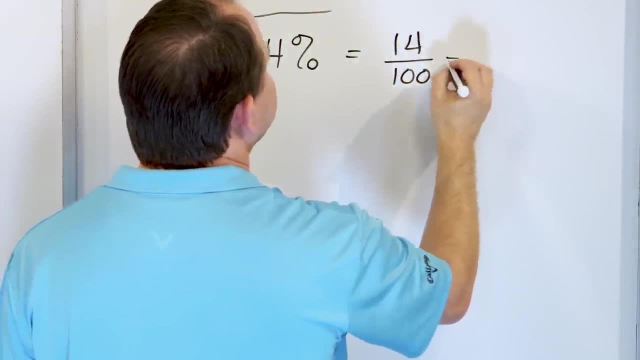 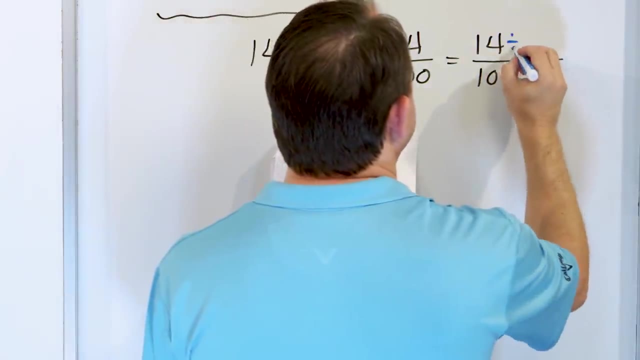 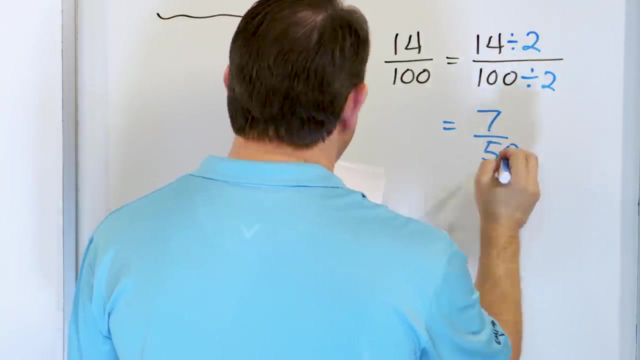 to a fraction: 14 over 100.. over 100.. These are both even numbers, so I can divide top and bottom by at least two. What do I get? 14 divided by two is seven. 100 divided by two is 50.. I get 7 50ths. This is the. 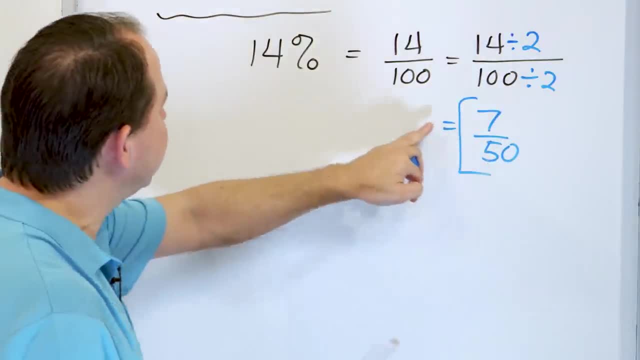 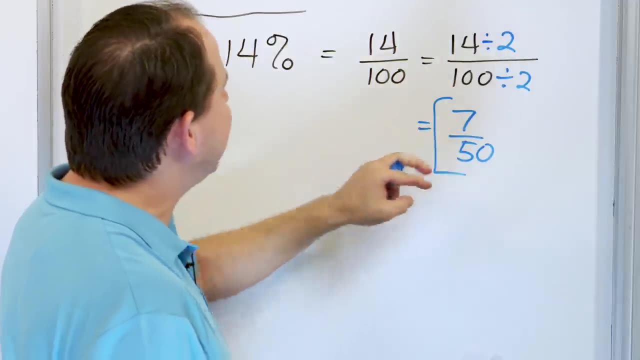 fractional equivalent of 14%. The numbers look totally different, but 14, as it compares to 100, is the same fraction as seven, or, when you simplify, is the same as 7 50ths. So these are equivalent. How do I convert this into a decimal? Well, if I'm dividing by 100,. 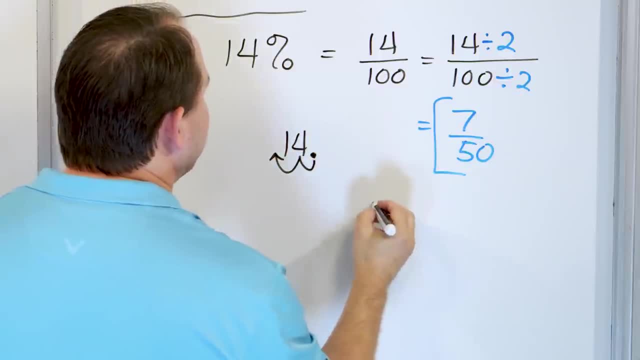 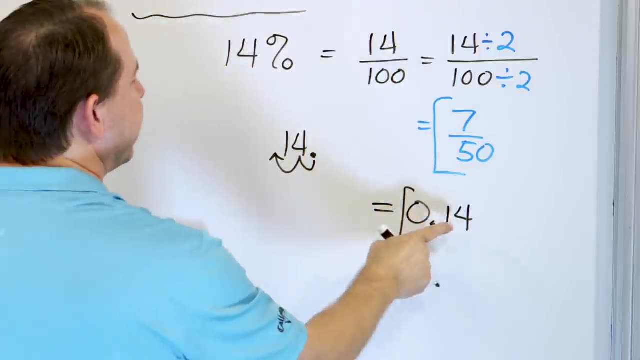 then I'm going to move that decimal two spots to the left, which means it's going to be 0.14.. So instead of doing the actual division, I just know I'm moving two spots to the left, So 0.14,. 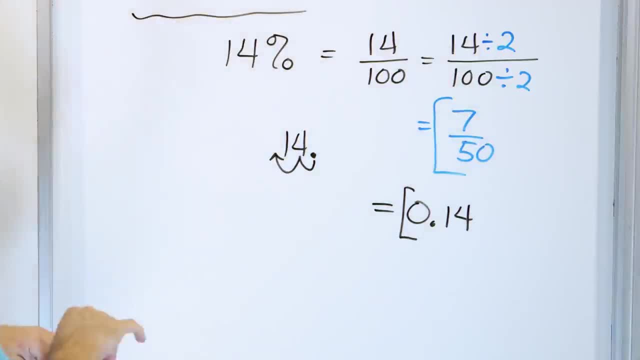 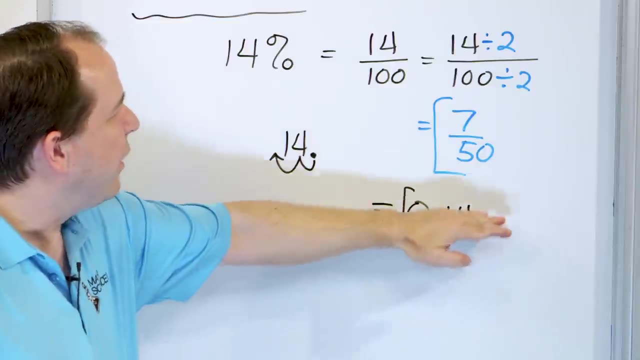 same as this and this fraction is the same as this. Notice that 11% and 14% are very small percentages, close to zero, So the decimal is also very close to zero. The fractions are also pretty small: 11 out of 100 or 7 out of 50, those are pretty small. 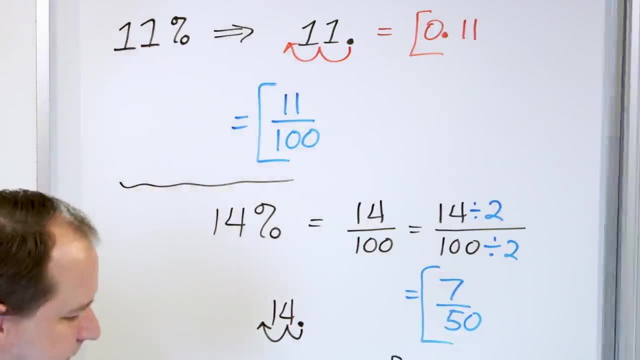 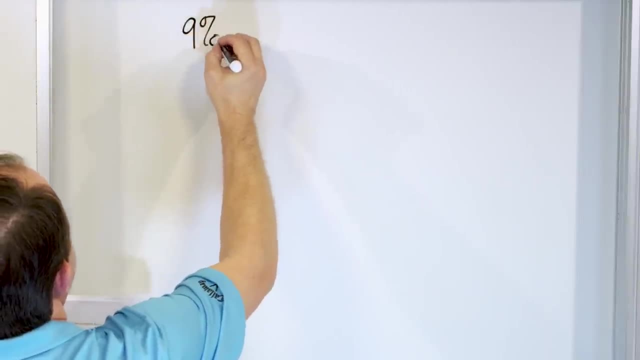 fractions, because the percentages are small in those cases. All right, we're on the home stretch. Let's take a look at 9%. How do I convert that to a fraction? Well, it's going to be 9 out of 100.. 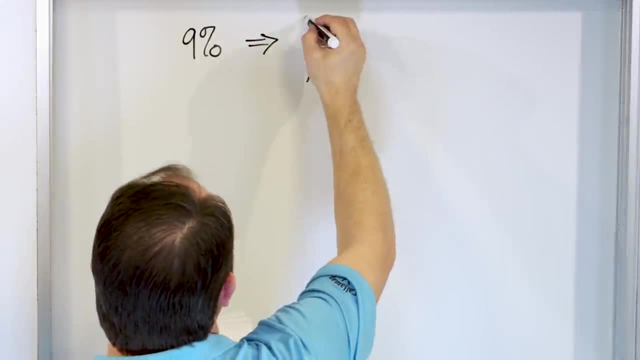 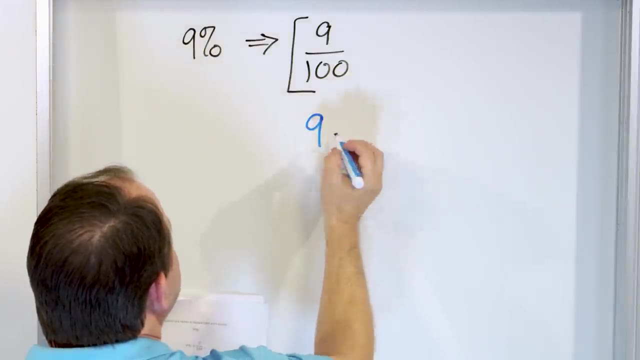 Can I simplify this? Actually, I can't. I cannot divide top and bottom and make it simpler. so this fraction is the same as 9%. How do I convert it into a decimal? Well, I'm going to take a 9,, which is a decimal point here, and I have to move it two. 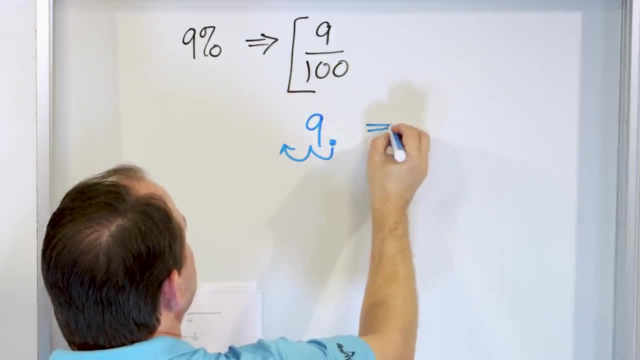 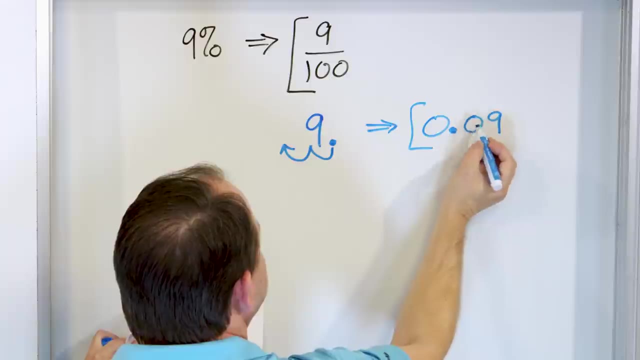 spots to the left. So I kind of have to insert a zero, making it 0.09.. This is the decimal, because if I started here and moved it two spots to the left, I have to insert that zero, So 0.09. 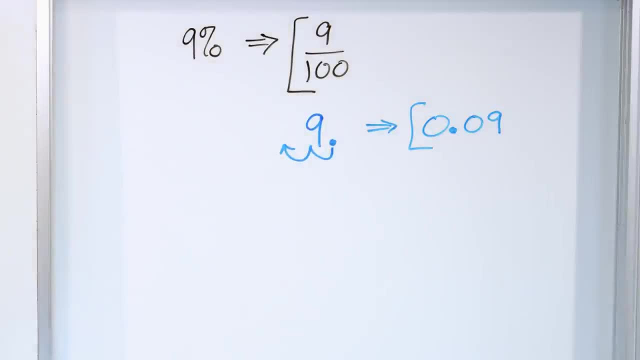 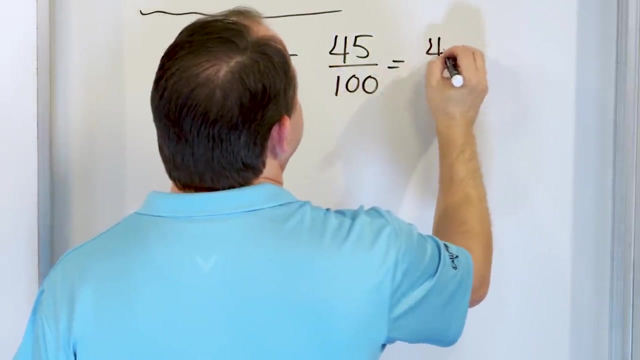 is the decimal equivalent and this is the fraction equivalent. All right, only a couple more. Let's take a look at 45%. How do I convert it to a fraction? 45 divided by 100, or out of 100.. So I'm going to simplify that as 45 out of 100.. And in order to 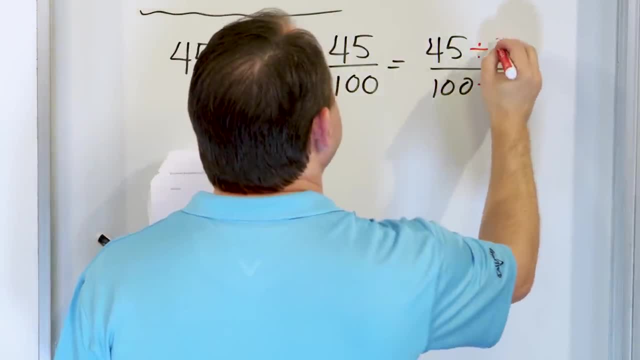 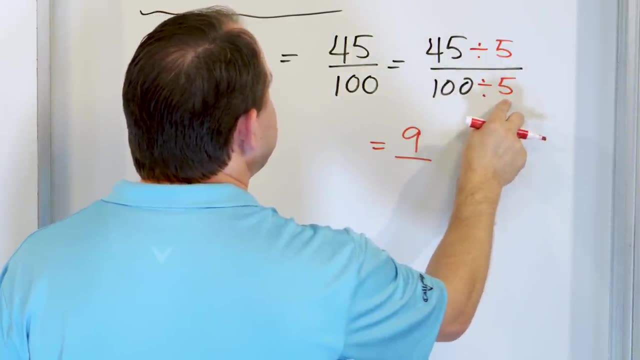 simplify that fraction, I'm going to divide the top and the bottom by 5.. They're both divisible by 5.. And so 45 divided by 5 is 9, and 100 divided by 5 is what? 20.. So the fractional equivalent to 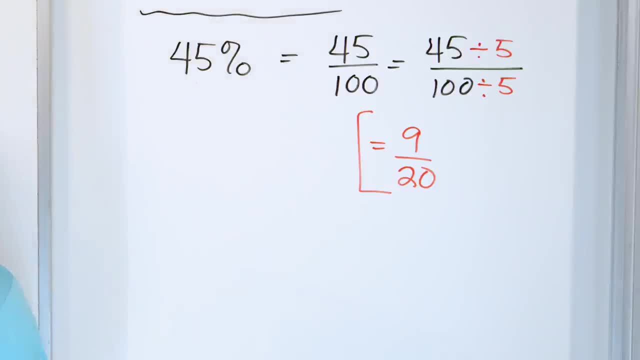 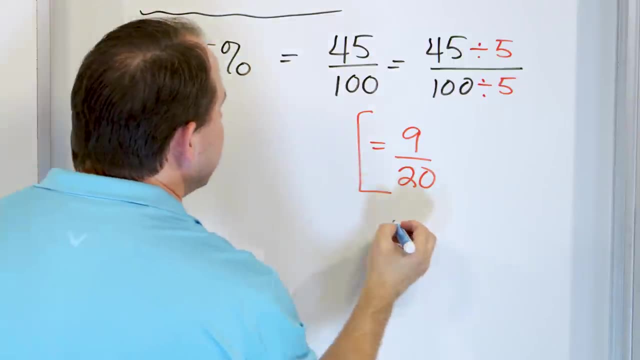 this percentage is 9 twentieths. What's going to be the decimal equivalent? By now you can see that there's a decimal here and you're dividing by 100.. All you're doing is moving it two spots to the left, So it's 0.45.. This is the decimal equivalent of that percentage, and here is 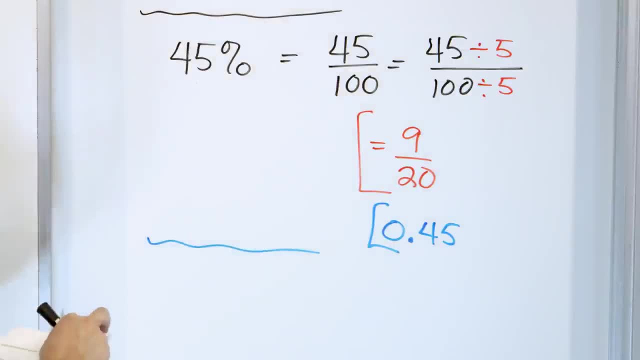 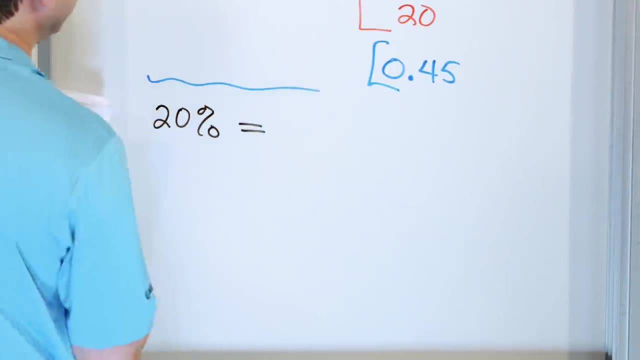 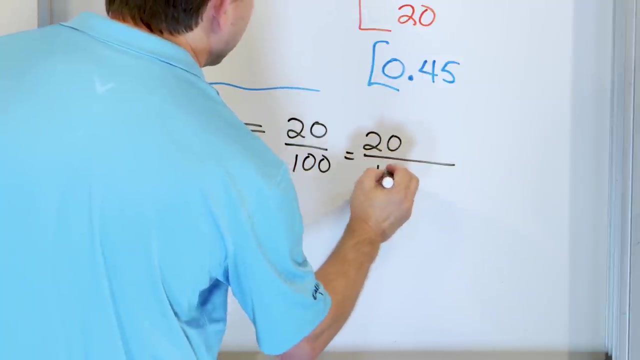 the fractional equivalent. All right, I think, only one more. Maybe there's two more. Let's take a look at 20%. How do I convert that to a fraction? 20 over 100.. And I can simplify this one: 20 over. 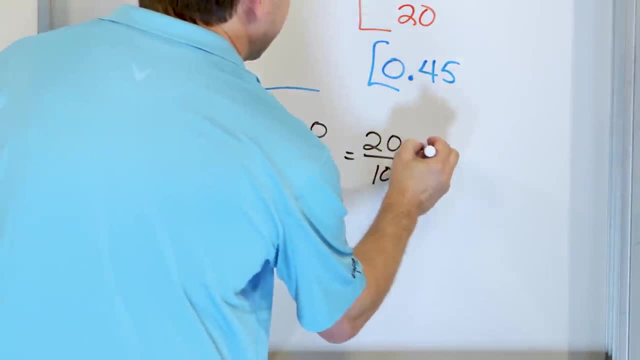 100.. I'm going to simplify: 20 over 100.. I'm going to simplify this one: 20 over 100.. I'm going to simplify it by dividing. I know I can divide by 5, but I can also actually divide by 20.. And so 20. 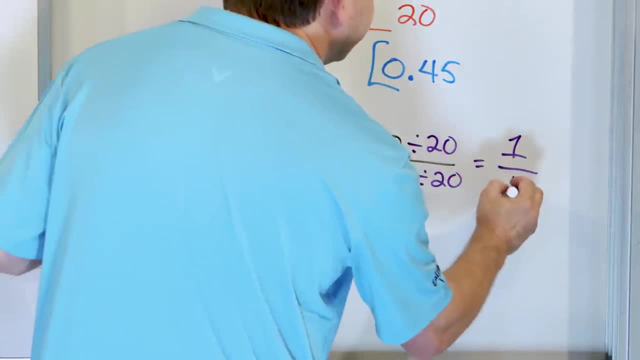 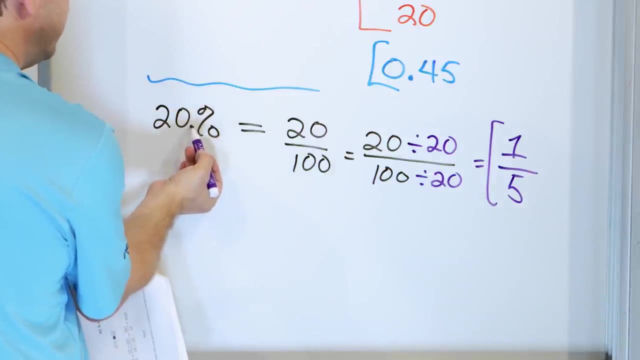 divided by 20 is 1, and 100 divided by 20 is 5.. So the fraction 1 fifth is the same as 20%. How do I get the decimal? There's going to be an invisible decimal here and I'm moving it two spots: 1, 2.. 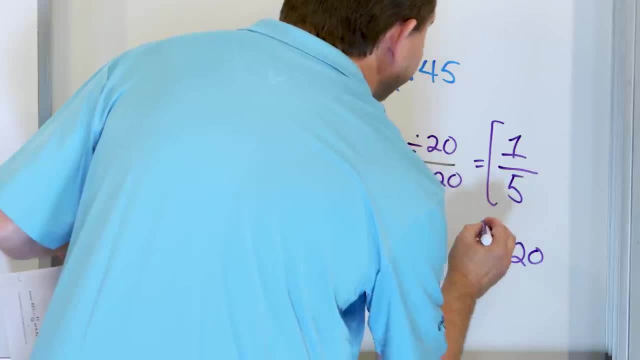 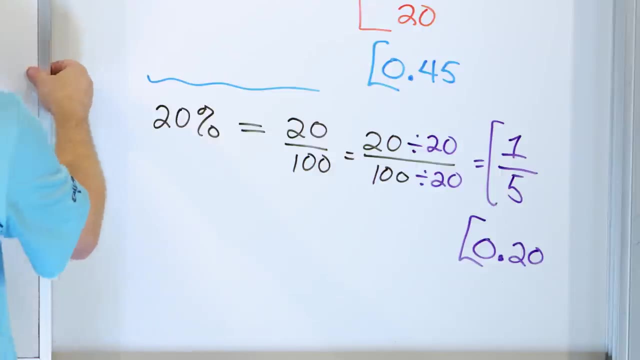 So 0.2.. Or you can write it as 0.20.. The trailing zero doesn't really do anything, and so you can write it as 0.2 or 1. fifth, Same thing. All right, let me do our last problem. I'll squeeze it in. 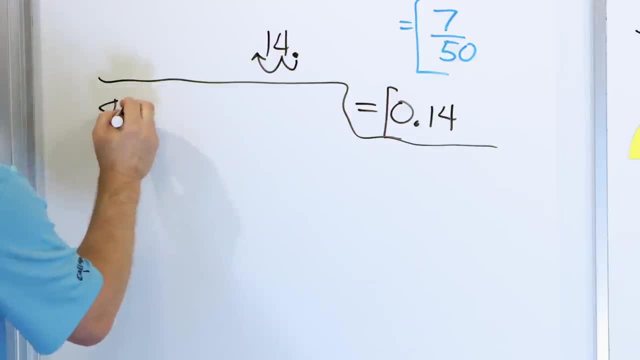 kind of over here. Last problem: 82%. How do I write it as a decimal? Write it as 82 over 100.. And I can simplify this because I can know I can at least be divisible by 2, right? So I'm going. 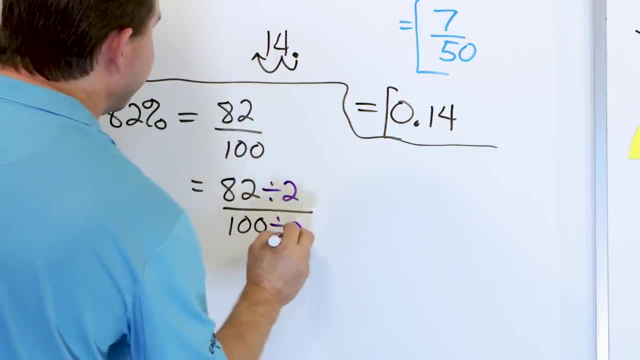 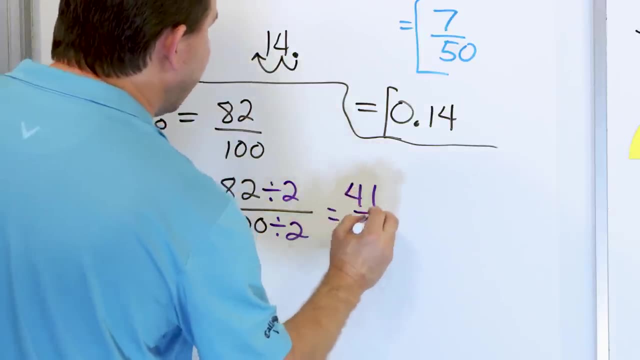 to divide top and bottom by 2. to simplify it: 82 divided by 2,. when you work through that 41,, you divide by 2, divide by 2, you're going to get 41, and 100 divided by 2 is 50. So 41 fiftieths. 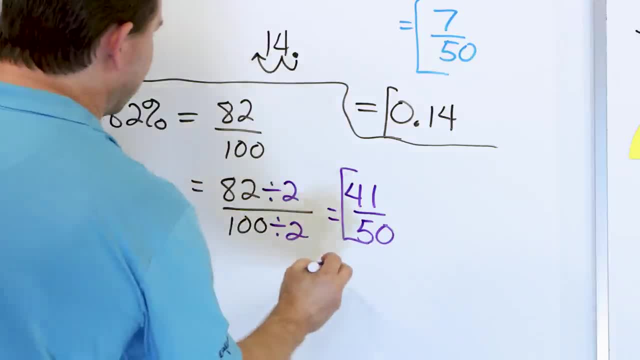 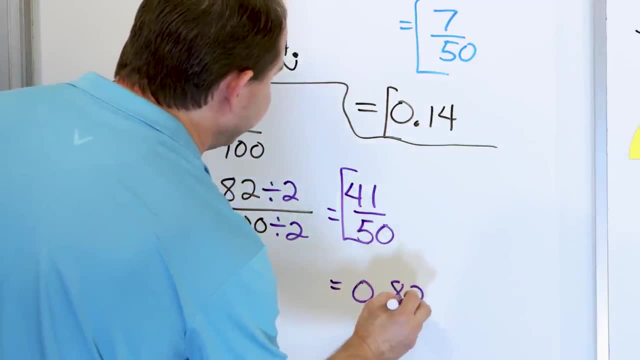 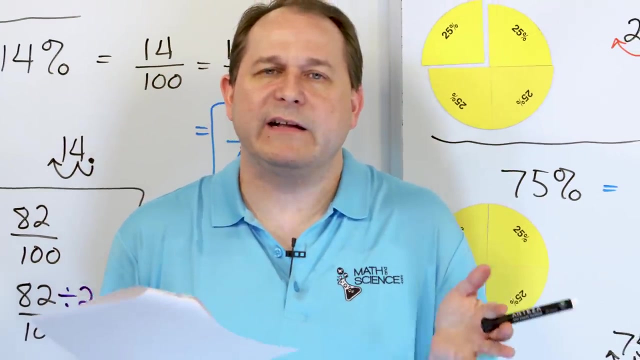 is the fractional equivalent of this And the decimal is. if I just know that there's an invisible decimal here and move it two spots to the left, 0.82 is the decimal equivalent. So here we have conquered what a percentage is, And we basically established that the percentage 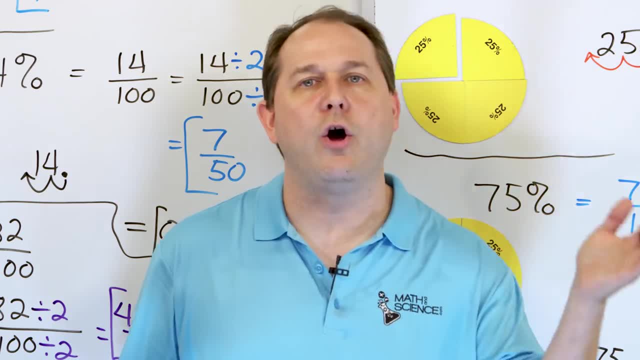 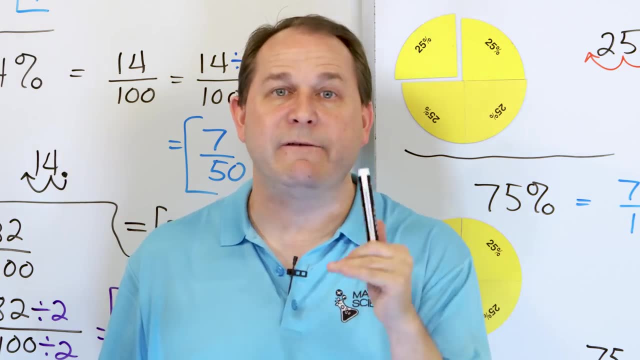 scale goes all the way from the low end of 0% all the way to the maximum of 100%, because it's a scale out of 100.. Right in the middle is 50%. That's when you give me half of something or there's a half of a chance of something happening.